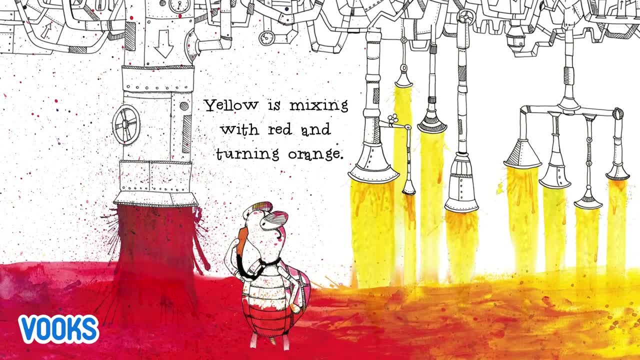 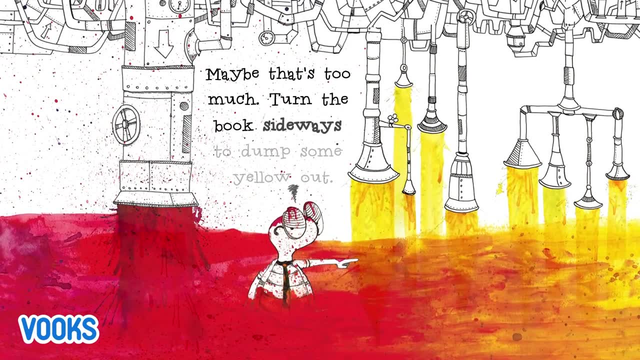 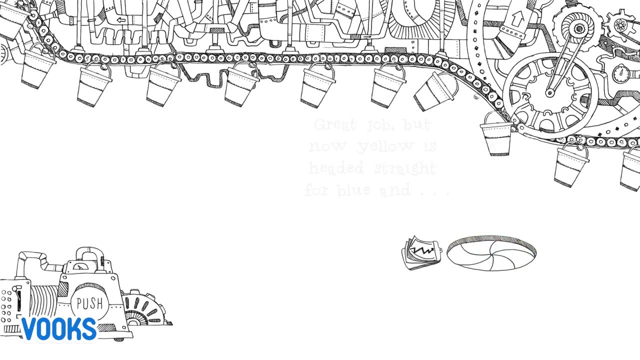 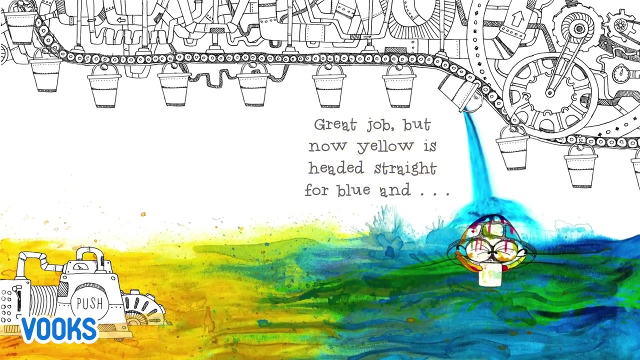 Yellow is mixing with red and turning orange. Hmm, Maybe that's too much. Turn the book sideways to dump some yellow out. Whoa, Great job. But now yellow is headed straight for blue and Whoa, and You guessed it. 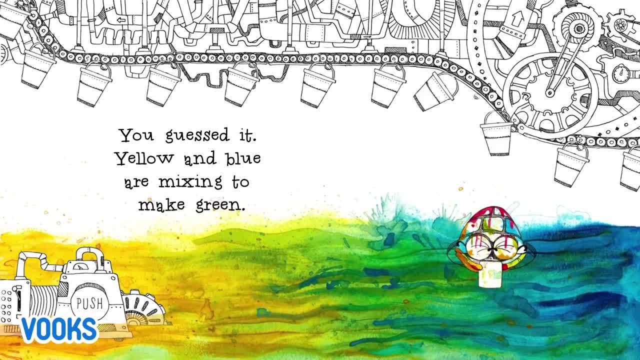 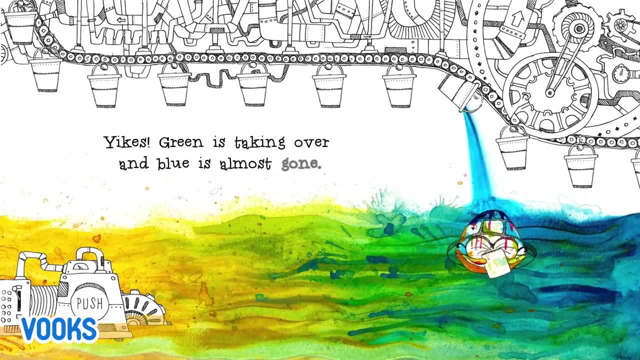 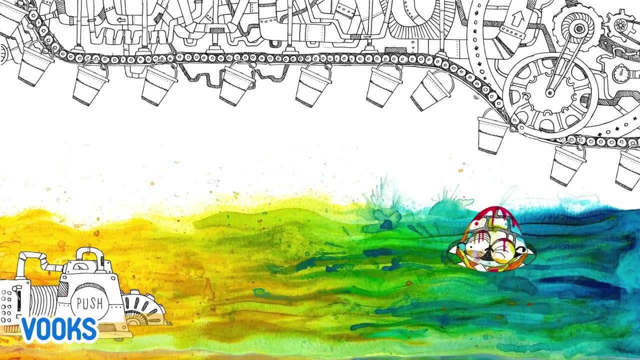 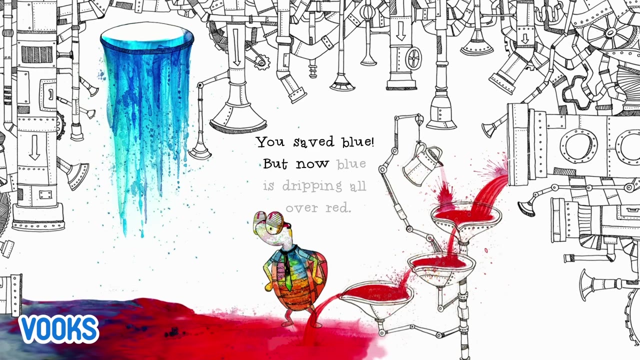 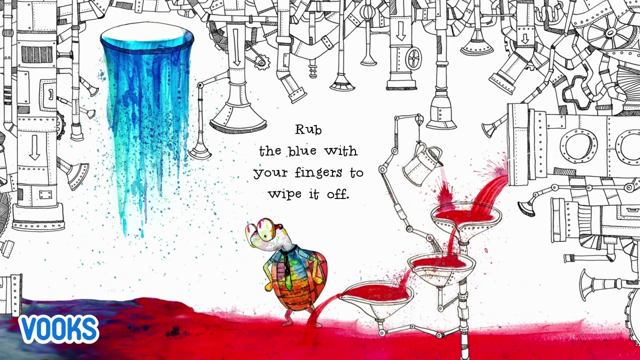 Yellow and blue are mixing to make green. Yikes, Green is taking over And blue is almost gone. Quickly push the button to drain blue. You saved blue, But now blue is dripping all over red. Rub the blue with your fingers to wipe it off. 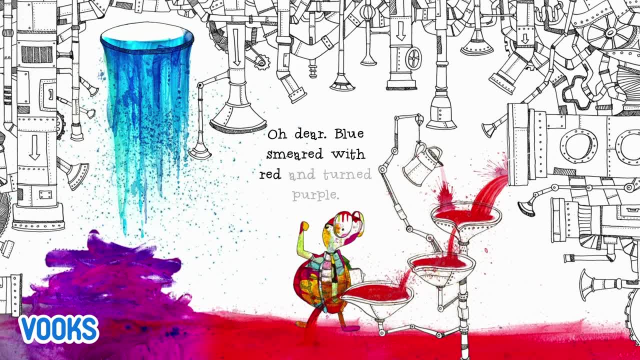 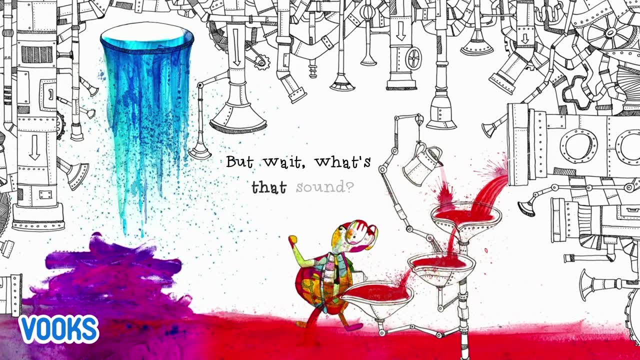 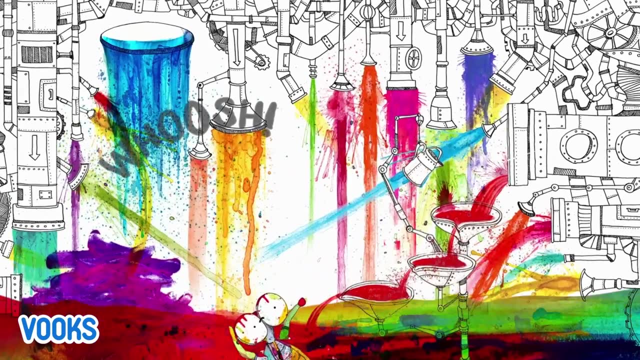 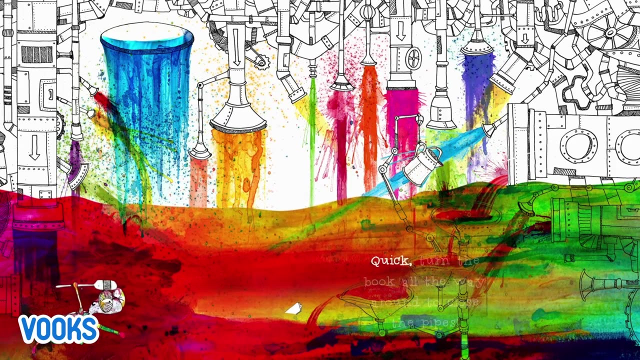 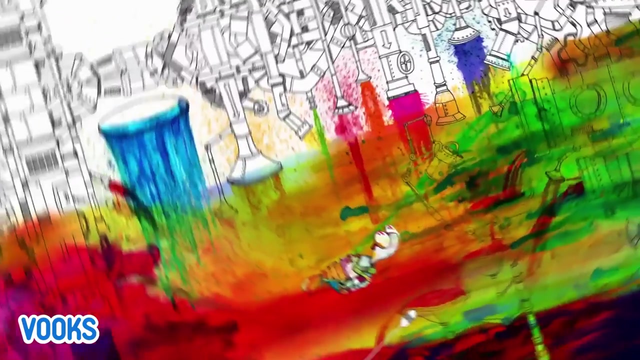 Oh dear. Blue, smeared with red and turned purple. But wait, What's that sound? Huh Whoosh, Splat, Huh Spray, Quick. Turn the book all the way around to close the pipes. Oh no, The pipes must be broken. 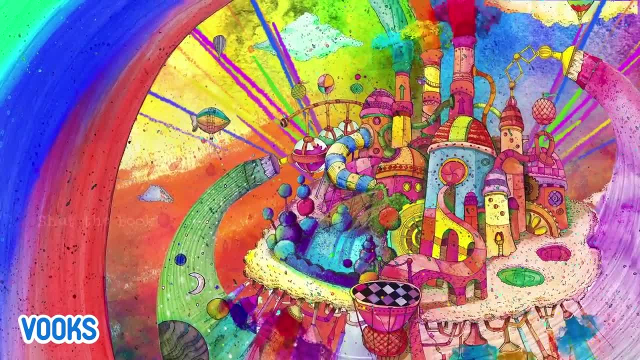 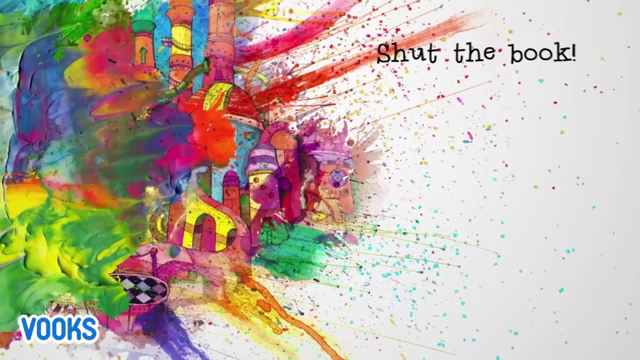 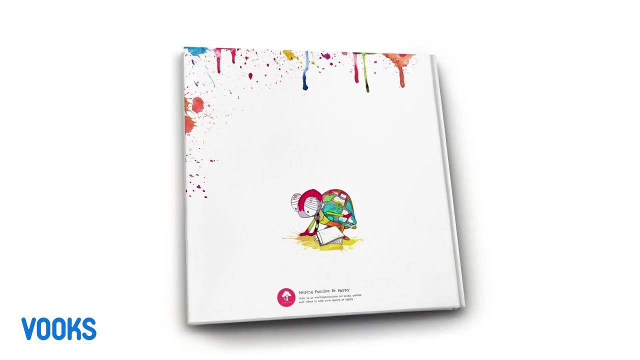 Colour's exploding everywhere. Shut the book One more time. Two, Three, Four, Five, Four, Five, Six, Seven, Seven On the count of three, Three. One more time: Four, Three, Four, Five. 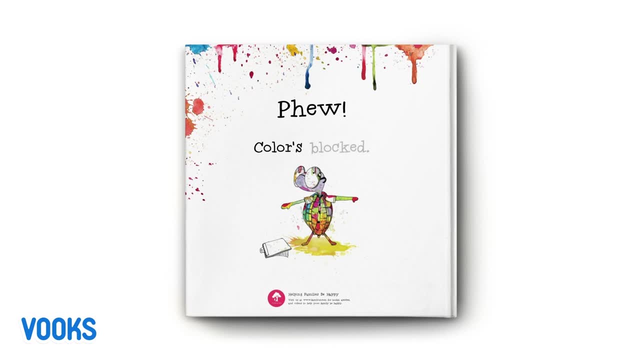 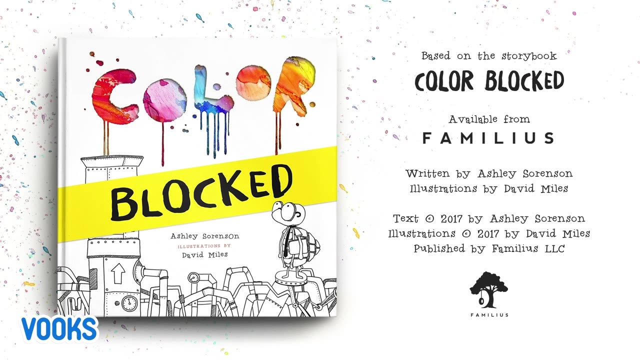 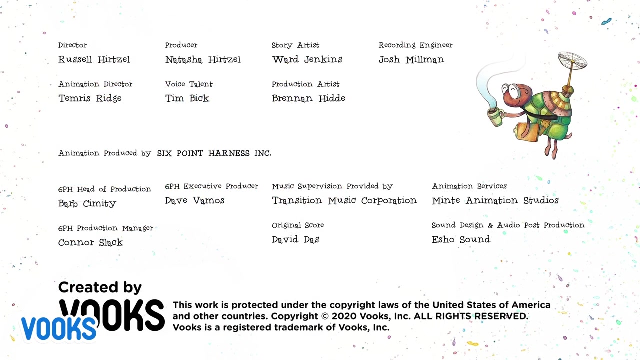 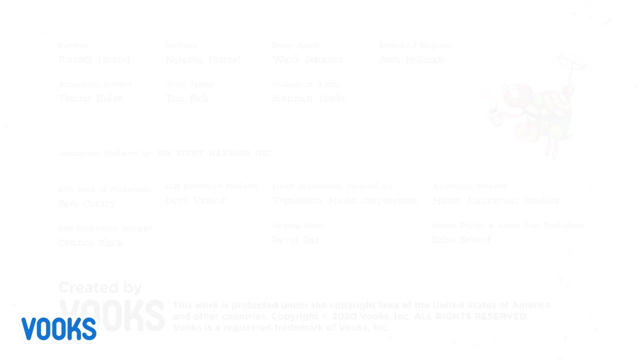 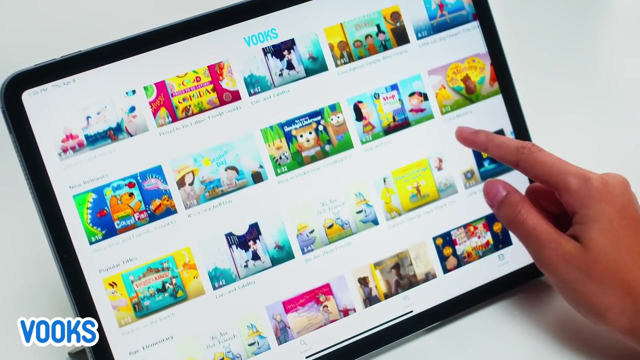 Four, Six, Seven, Six, Seven, Eight, Seven. Here we go. If you don't have books, then what are you waiting for? Books is kids safe. it has storybooks that are brought to life and third, it's fun.